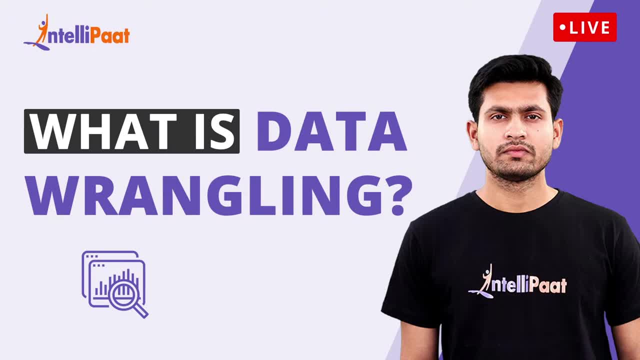 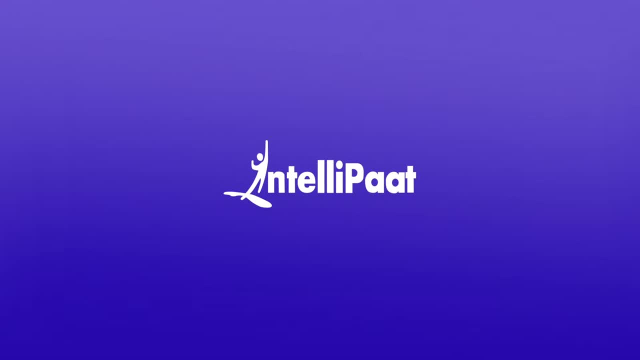 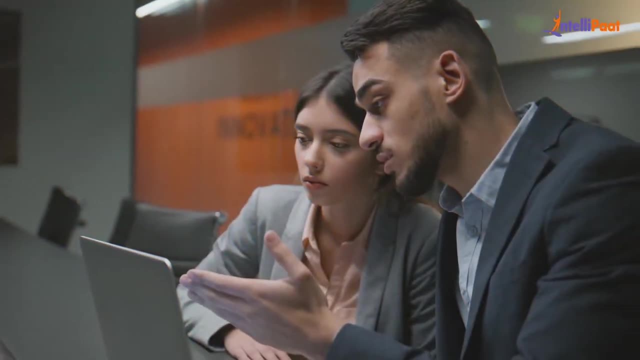 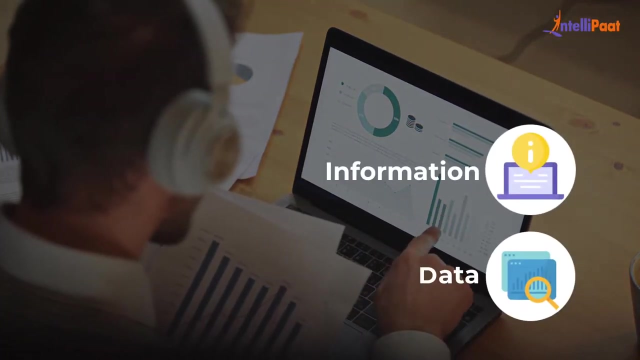 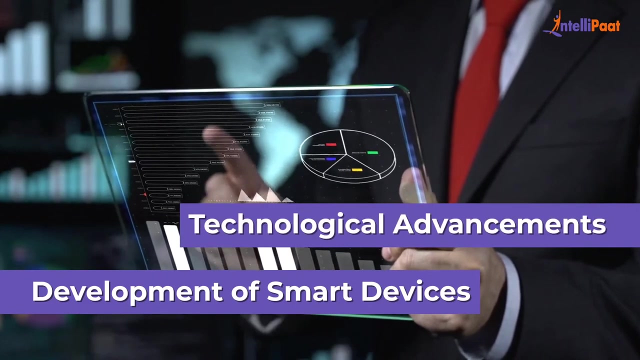 Hello everyone and welcome to today's session on what is data wrangling. Do you know, friends, that businesses have long relied on data scientists and analysts to understand and leverage the information and data? The proliferation of data as a result of development of smart devices and other technological advancements has accelerated. 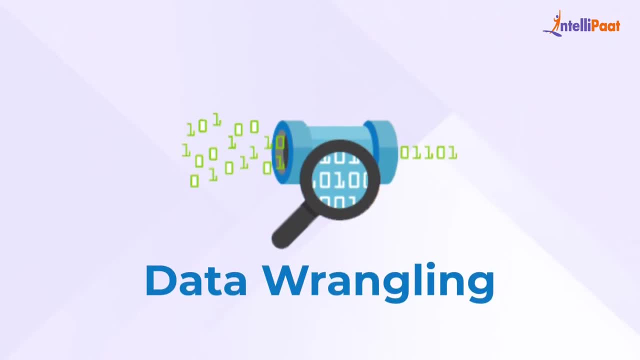 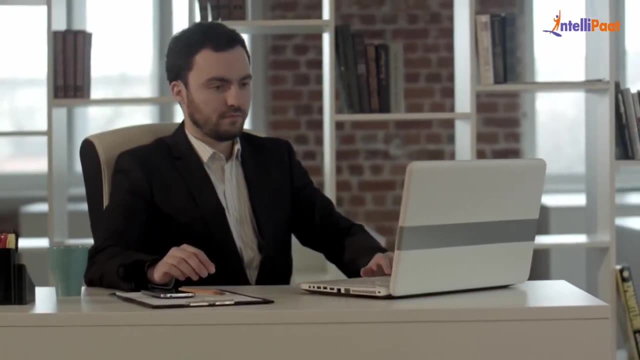 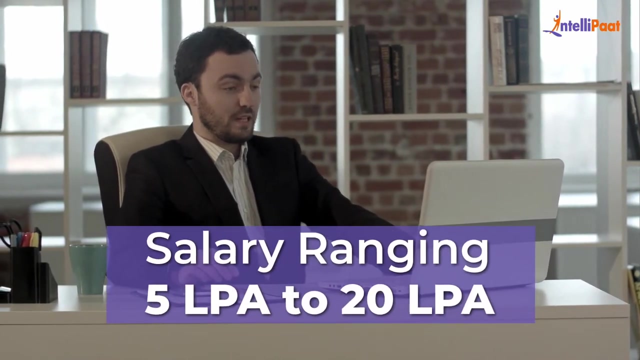 this need. After learning certain skills like data wrangling, SQL, Python, Excel, Power BI and many more, you can get a good, high paying job, such as business tragedy analyst, data analyst, etc. with a salary ranging over 5 LPA to 20 LPA. Now, before we hit on our today's agenda, 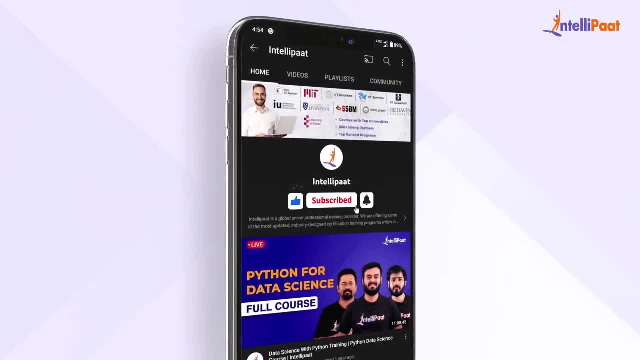 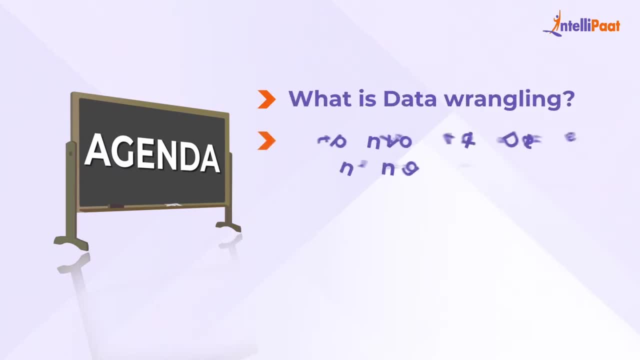 do not forget to hit the subscribe button. So first we are going to be starting with what is data wrangling, Then we are going to discuss about steps involved in data wrangling. Moving ahead, we are going to learn about getting started with Python libraries and at the end, we are going to conclude our session with 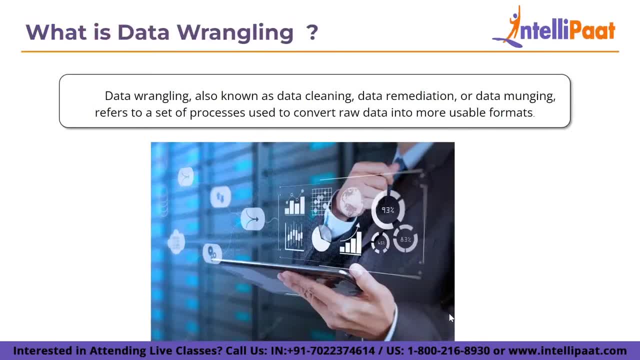 a good hands on. So let's start with. what is data wrangling? Data wrangling, also known as data cleaning, data remediation or data munging, refers to a set of processes. It is used to convert raw data into more usable formats. The exact methods vary depending 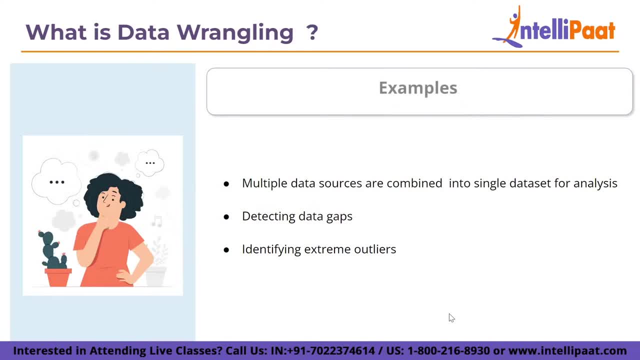 on the data you are leveraging and the goal you are attempting to achieve. Here are some of the examples of the data wrangling. For example, you have multiple data sources that are combined into a single data set and that is used for analysis. So that comes under data wrangling. Or you can do such as you. 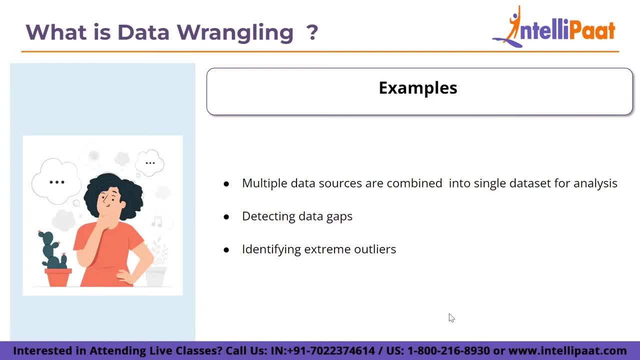 can detect data gaps Or you can remove the data that is unnecessary or irrelevant to the project at hand, Either explaining or identifying extreme outliers in the data, and either explaining or removing them so that data analysis can be proceeded. Data wrangling can be done manually or automatically When dealing with extremely large data sets. 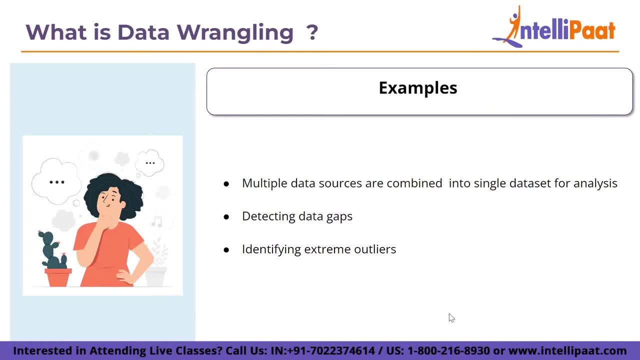 automated data cleaning can become kind of essential. Next or other team member is usually in charge of data wrangling. in an organizations that have full data team, Non-data professionals are frequently in charge of cleaning data before leveraging it in small organizations. Now we will look at steps that are involved in data wrangling. 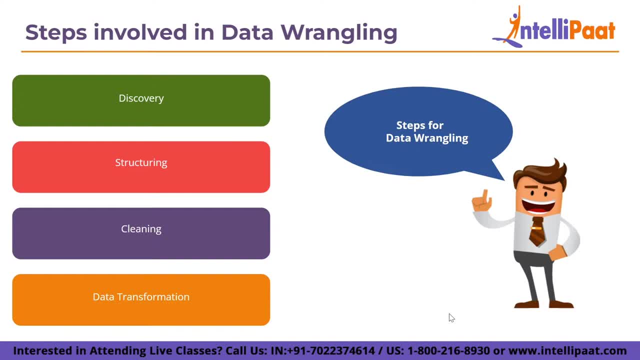 To ensure that final data set is reliable and accessible, each data project necessitates a distinct approach. Having said that, The approach is typically informed by a number of processes. These are also known as wrangling steps or activities, And the first such is called discovery, In this process of becoming acquainted with the 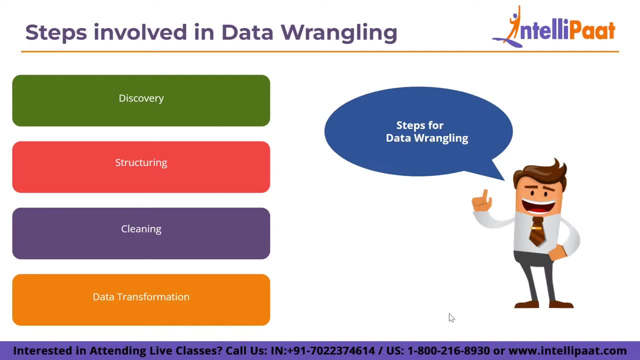 data in order to conceptualize how you might use it is referred to as, basically, discovery. It's similar to checking your refrigerator before cooking a meal to see what ingredients you have on the hand. During the discovery process, you may notice trends or patterns in the data, as well as obvious issues such as missing or incomplete values that must 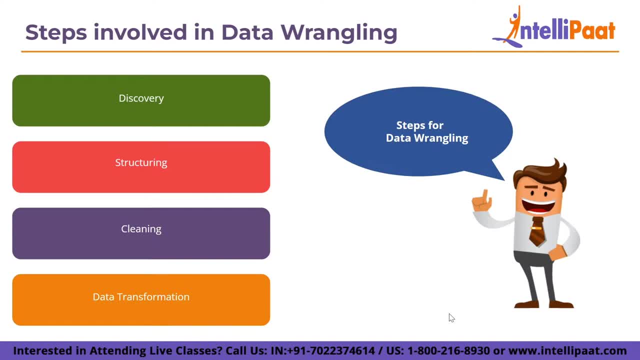 be addressed. This is an important step because it will inform all subsequent activities. Next is structuring. In structuring, basically, raw data is usually unusable in it's raw form because it is either incomplete or incorrectly formatted for the intended application Data. 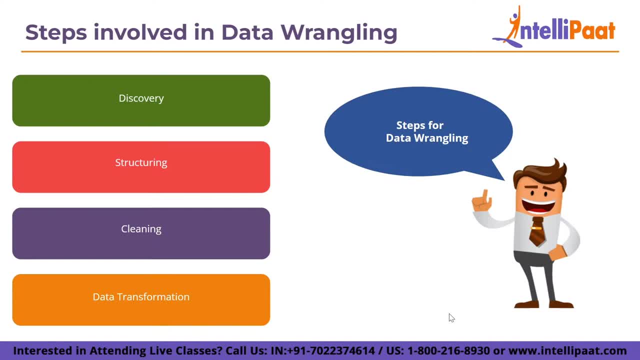 structuring is the process of transforming raw data to a data base. Data structure can be anything anywhere from data to data. Data is a process of processing data, data, Data, raw data- so that it can be more easily leveraged. The format of your data will be determined. 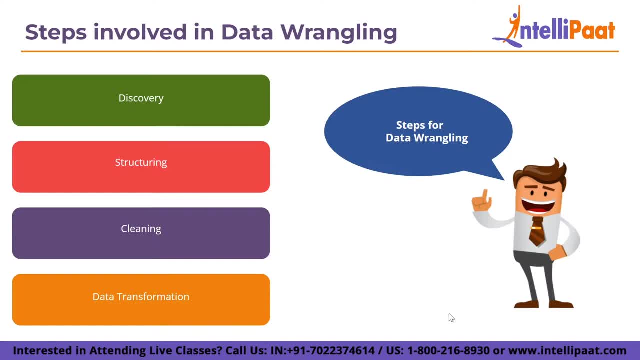 by the analytical model you use to interpret it. Next step is called cleaning. Data cleaning is the process of removing inherent errors in the data that may distort or diminish the value of your analysis. Cleaning can take up many forms, such as removing empty cells or rows, removing outliers and standardizing. 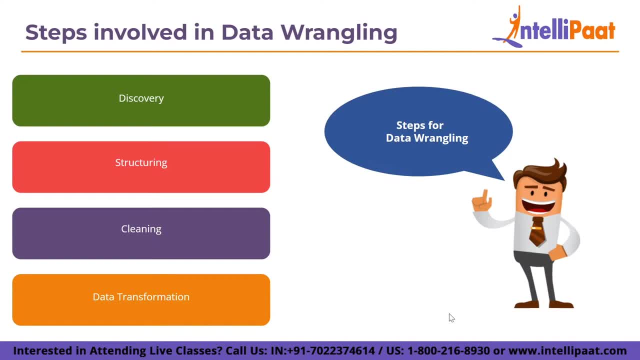 inputs the goal of the data that could affect your final analysis. In the cleaning of data, there are lot of processes or tasks involved, such as it can be changing the name, sorting and rearranging, conversion of data types or data duplication, addressing missing or 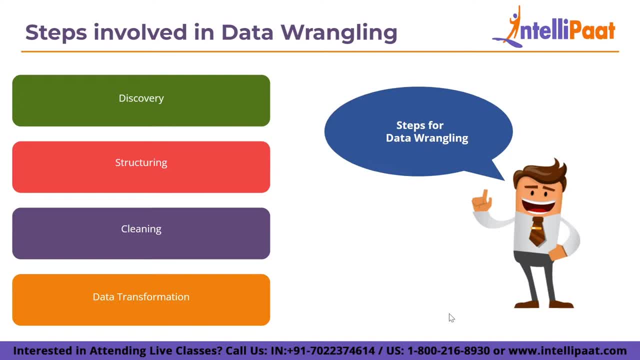 incorrect data filtering data to be desired. subset Data cleaning is also the best place to start when it comes to data wrangling, because, having the data stored in the correct data type, the data could be restricted to the data being stored in different types of data. 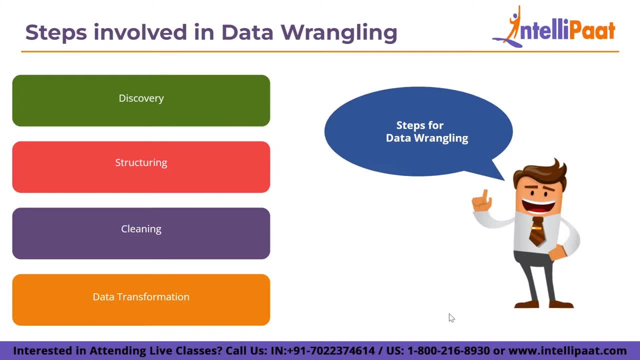 types with easy to reference names is kind of easier to go for. Next step is called data transformation. Often we will arrive at the data transformation stage after some initial data cleaning, but it is entirely possible that our data set is unusable in its current form and that we 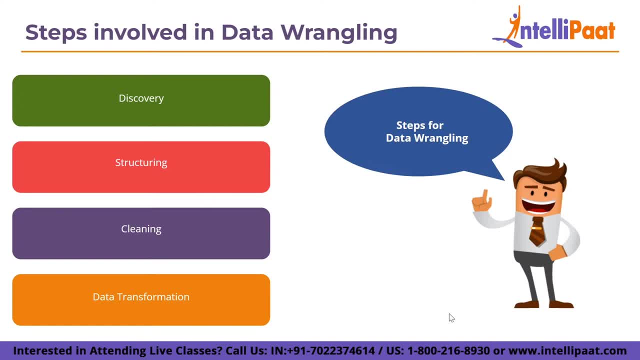 must restructure it before attempting any data cleaning. We focus on cleaning the structure of our data to facilitate downstream analysis. in the data transformation, This usually involves changing which data goes along the rows and which goes down the columns. The majority of the data we will find is in either a wide or a long format. Each of these formats has the advantages and 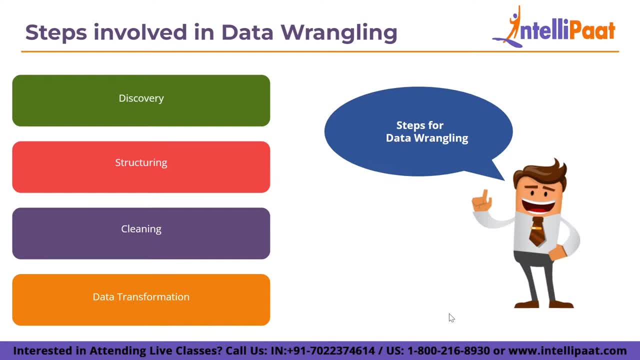 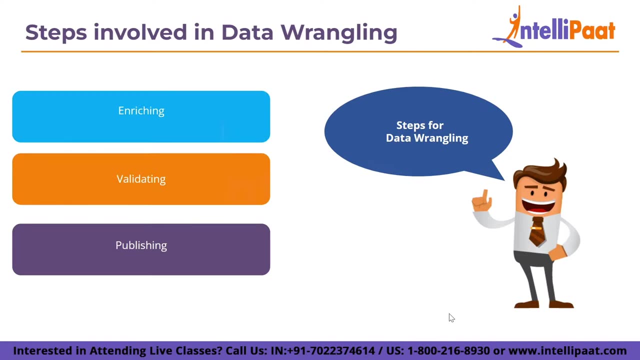 disadvantages, and it's important to know which one we will need for our analysis. People frequently record and present data in the wide format, But certain visualizations also require the data to be in the long format. Now let's look at to the next process. The next step is called enriching, Once you have analyzed your existing data and 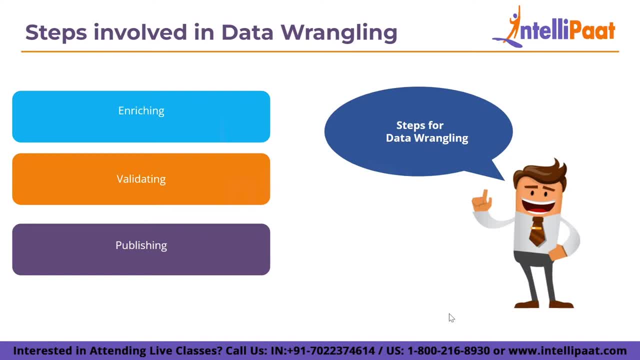 transformed it into something more usable. you must determine whether you have all of the data required for the project at hand, And then we want to enrich the data. We can either merge new data with the existing data by appending new rows or column, or use existing data to generate new data Using the original data. we can improve our data in the 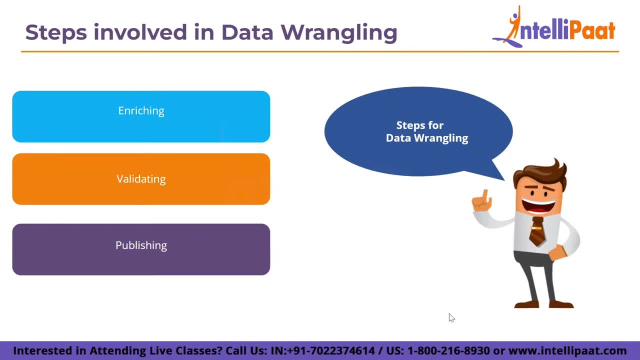 following ways, such as we can add new columns, use functions on the existing columns or data to generate new values. Next process is called binning. In this process we can also use the continuous data or the discrete data with the distinct values into a range of buckets which 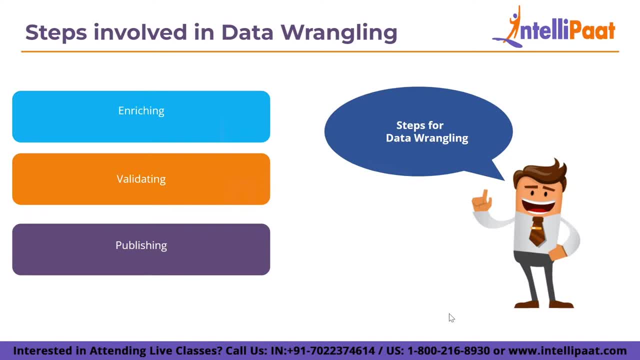 discretizes the column while allowing us to control the number of possible values. The next step we can do is called aggregating, which is basically means compiling and summarizing the data. The next what we can do in enriching the data is resampling in this process of aggregating. 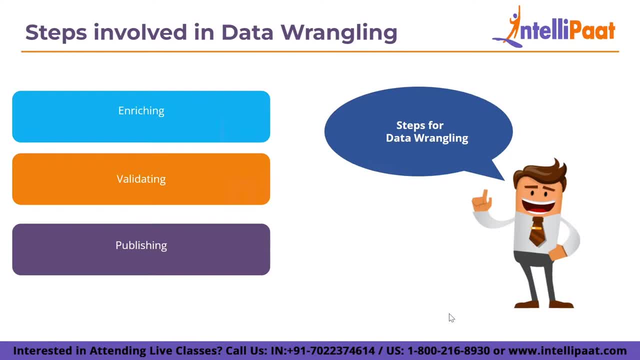 the time series data at regular intervals. Now let's look at the next step. that is called validating. So, basically, data validation is a process of ensuring that your data is both consistent and of sufficient quality. You may discover issues that need to be resolved during validation or conclude that your data is ready to be. 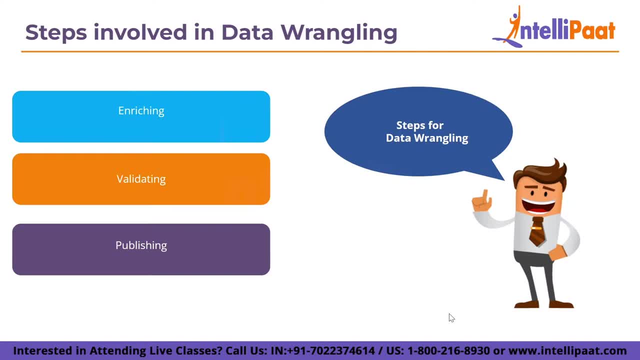 analyzed. Validation is typically accomplished through a variety of automated processes that necessitates programming. Next is, and the final step is called publishing. You can publish your data once it has been validated. This entails making it available for the analysis to the others within your organization The format in which we share your information. 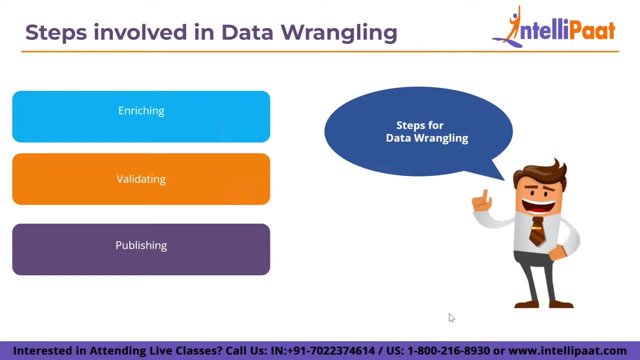 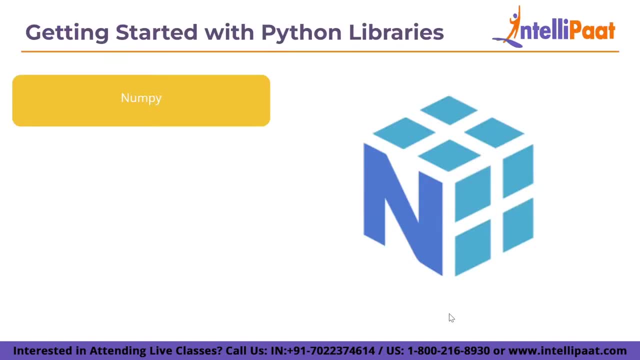 such as a written report or electronic file, will also be determined by the data and the goals of the organization. Now let's look at the next topic, which says that, getting started with Python libraries, The first one is called NumPy, So basically, NumPy is an abbreviation. 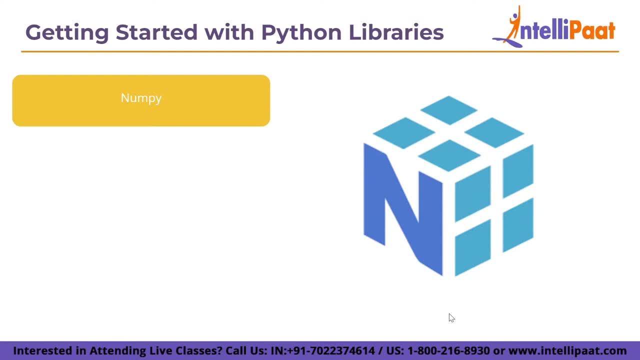 for numerical Python. It is the most important library. Python also has a scientific library for dealing with multi dimensional arrays, matrices, methods for computing. It is the most efficient library for efficiently computing mathematical problems. Next library we are going to discuss is called Pandas. Pandas is basically a data exploration. 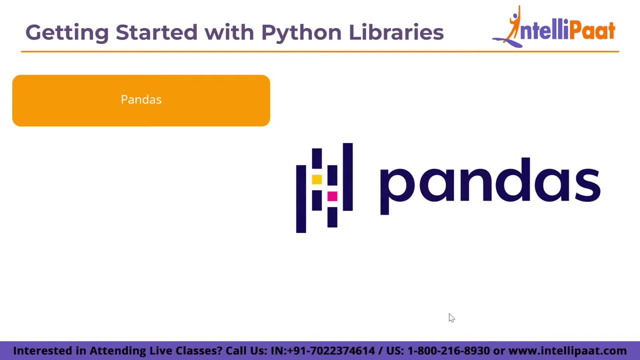 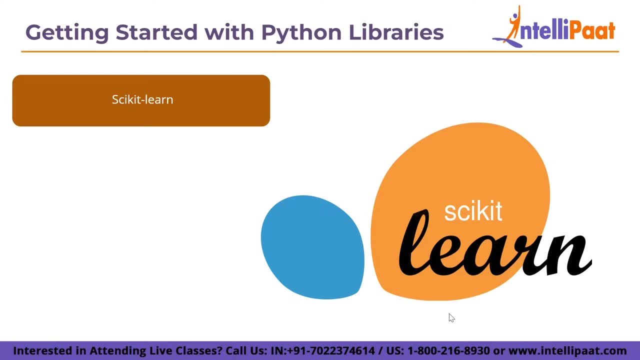 and a manipulation library that provides tabular data, data structures such as data frames, and various data analysis methods and manipulation. Next is scikit learn. Basically, if I talk about scikit learn, it is an acronym that stands for scientific toolkit for machine. 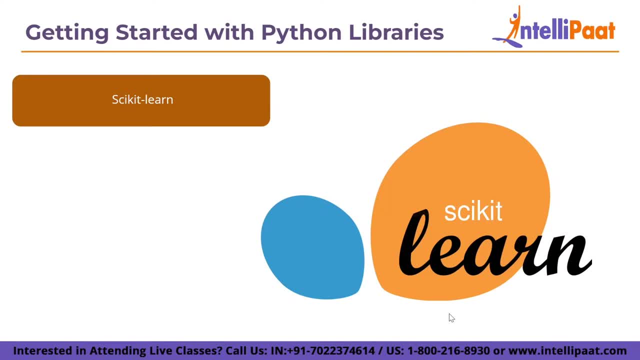 learning. It is a multi dimensional library and it is a very, very important library for machine learning. It is a machine learning library that provides supervised and unsupervised learning. methods such as regression, classification, dimensionality reduction and clustering are 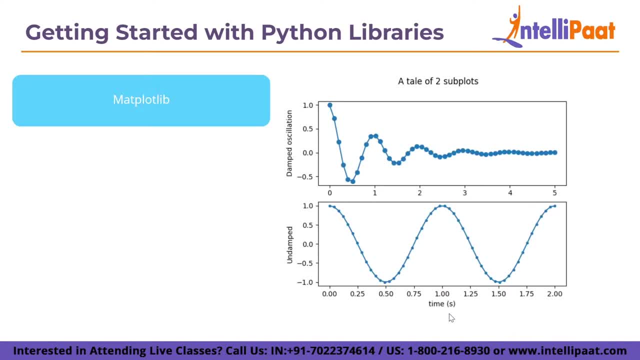 few of the examples of this algorithm. Next library we have it's called Matplotlib. This is basically a fundamental data visualization library that serves as a foundation for all other python visualization libraries. It provides 2d and 3d plots, graphs and charts. 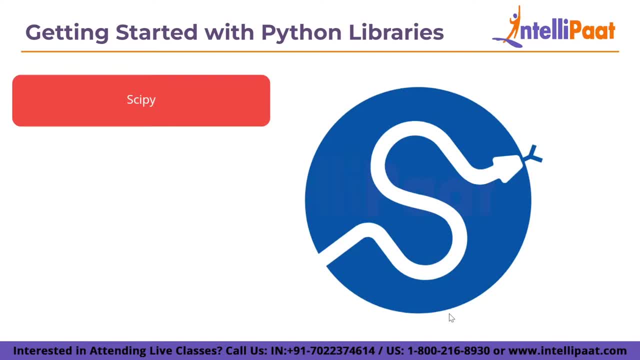 and also graphs for data exploration. It is built on, basically, NumPy and SciPy. Let's look on to the next library, which is SciPy. This is actually the powerful scientific computing library for performing calculations, operations in science, mathematics and engineering. 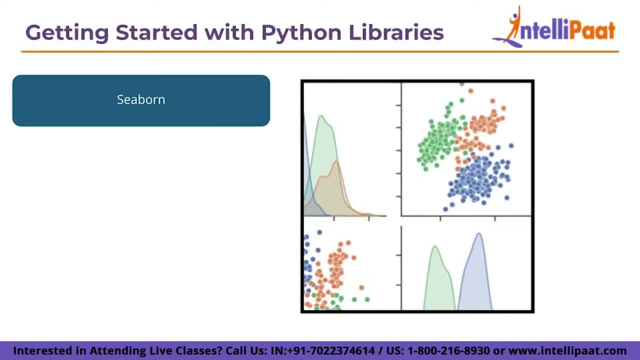 Let's look on to the next library we have. This is Seaborn. Seaborn is based on Matplotlib and provides high-level easy-to-draw visualizations. The plots are more interactive and well-organized, And our final library is Plotly. 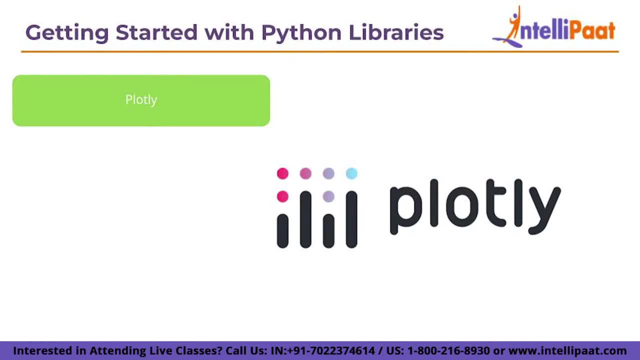 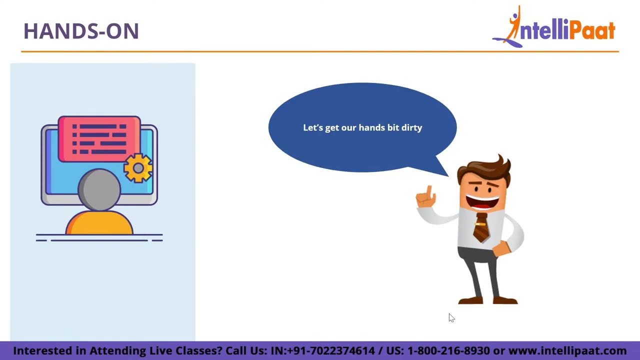 Plotly if I talk about is a library for data visualization. It provides high-quality interactive content: scatter charts, line charts, bar charts, histograms, box plots and other subplots and heatmaps. Yes, you guessed it right: We are going to do some hands-on thing on data wrangling. 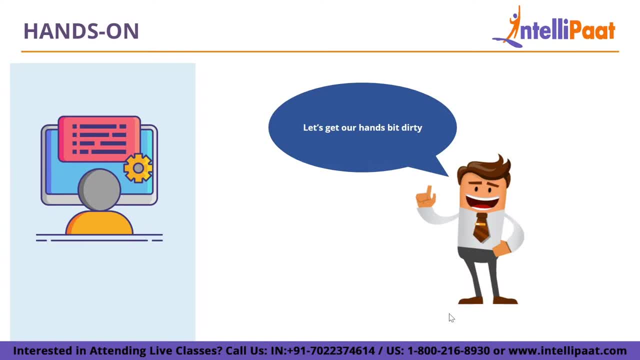 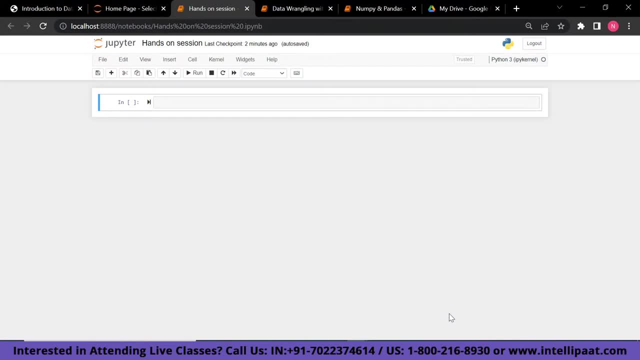 So we are going to basically take a data set and put it on a plot And we are going to perform few of the operations. So, without further ado, let's get into that. So now we will do some hands-on session. 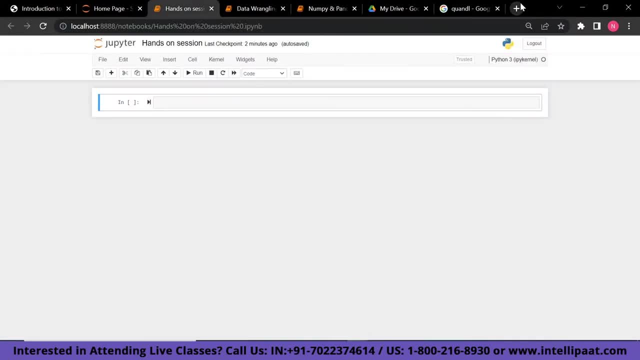 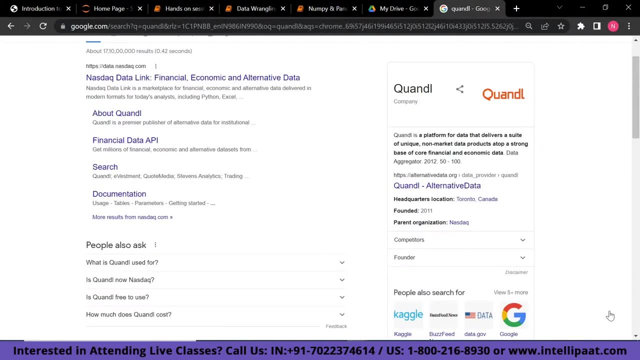 Now, before I do and upload the data set, I want to tell you about something. There is a company called Quandl, So basically now we will be working with the Quandl data set. Quandl is basically a Canadian firm that provides commercial and alternative financial data to the investment analysis. 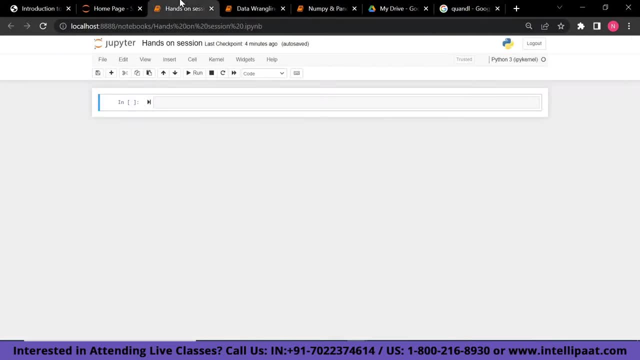 Quandl recognizes the investment analysis, So Quandl recognizes the importance of investment and financial quantitative analysis. Now let's see. Let's see how to query data in a Pandas data frame. Obviously, the first step would be to download the data. 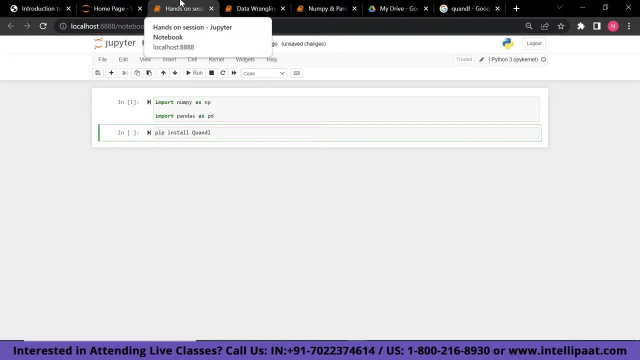 So we are going to use some codes all over here, But first let's import Pandas and NumPy. So, as you can see all over here, we have imported NumPy and Pandas. Now we are going to install the Quandl data set. 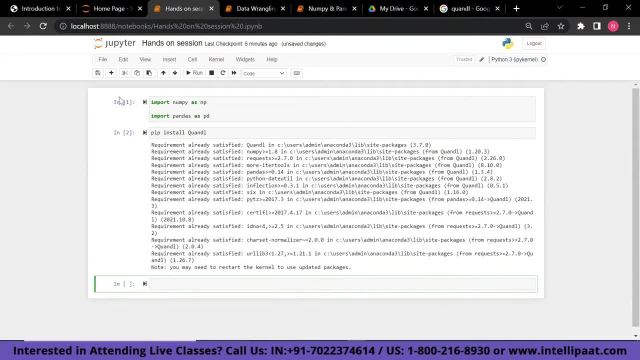 So, for the same, I'm going to run the cell And the data set is going to get uploaded. Now I have installed the Quandl data set. The next step we are going to do is we are going to import the Quandl data set. 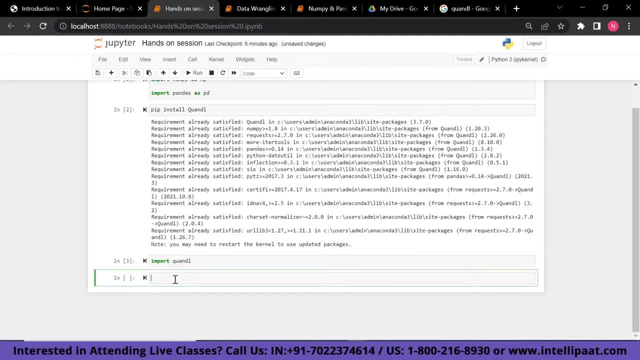 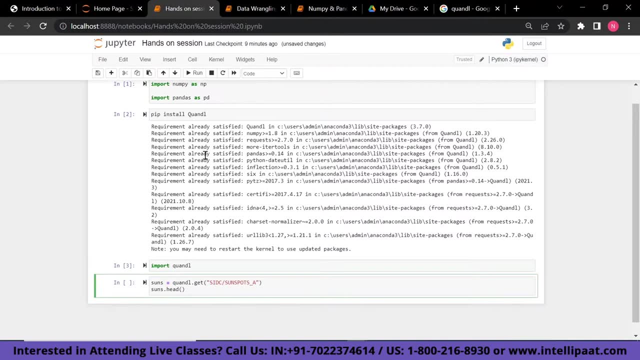 So I have typed import: Quandl. Now let's run the cell. Now our Quandl data set has been uploaded. Now I have created a variable called suns, Where I'm trying to access the sunspot data from the Quandl data set. 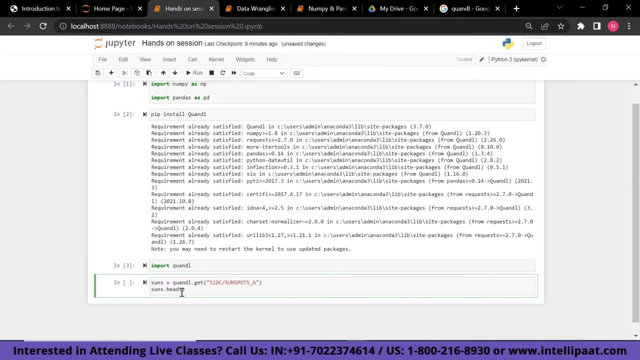 Okay, And then I'm trying to print sunshead. So basically, if I talk about head and tail functions, these methods serves for the same purposes as corresponding in the Unix commands: Choose the first and the last and records of a data frame. 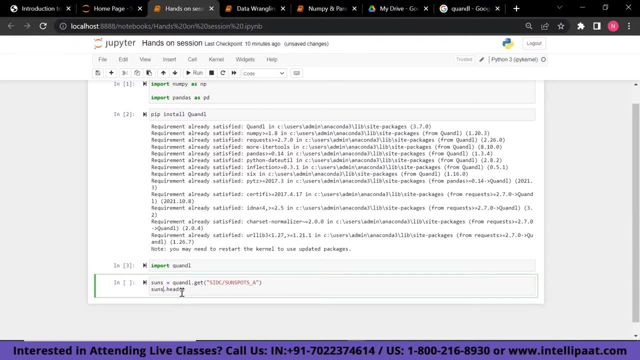 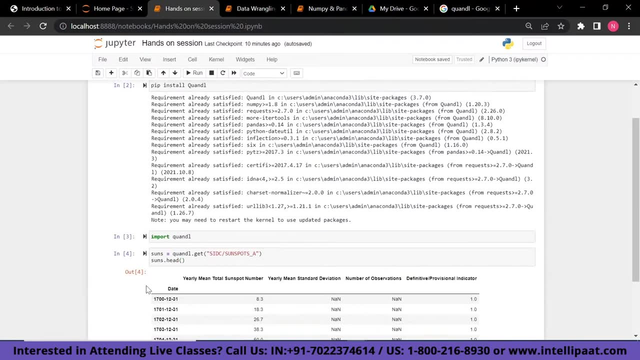 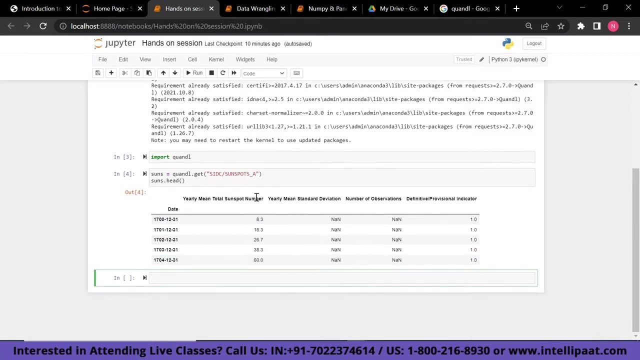 Where n is basically any kind of integer. So the head and the tail methods give the first and the last five rows of the sunspot data respectively. Now let me run the command So you can see. we have the first five records all printed all over here. 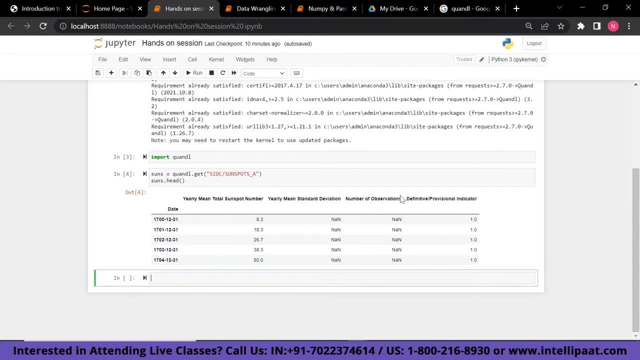 So we have date, We have yearly mean total sunspot number, We have yearly mean standard deviation, We have number of observations. Then we also we have a column with a name: definitive or provisional indicators. You don't have to worry about what these columns means. 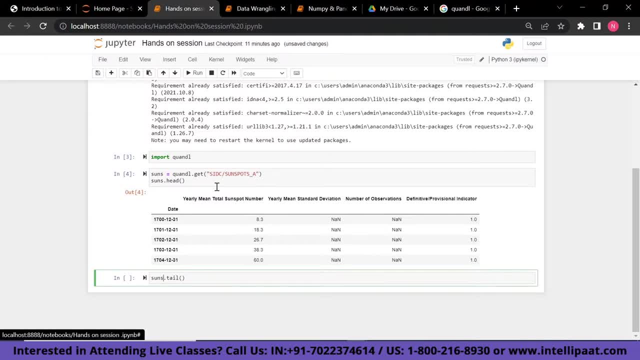 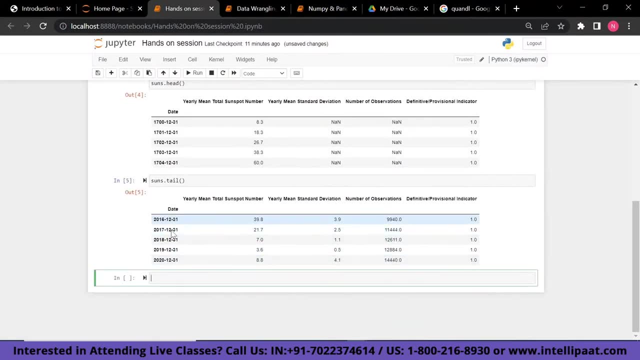 Just know and get aware about what these columns stands for. Okay, let's move further. So, since we have done the head, now it's time to run the tail. So you can see, we have received the last five records. Now let's move further and try to do some other operations. 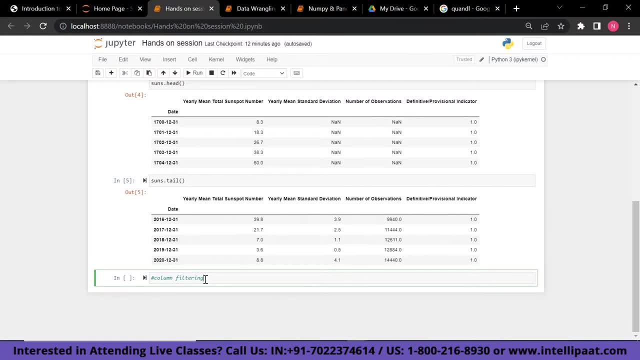 Now the next thing, what we are going to do here, is we are going to perform the column filtering. So basically, Panda supports column selection and that's look at some of the columns in the Pandas data frame. So basically, when we are trying to filter the columns, 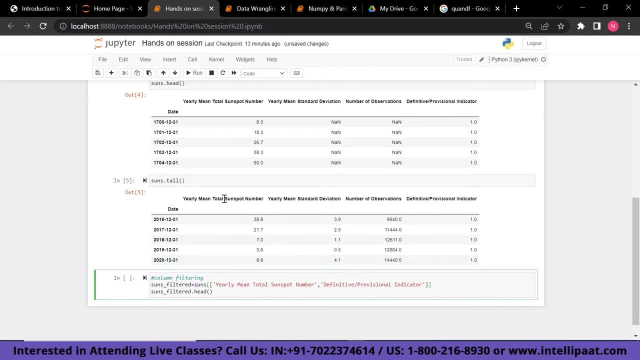 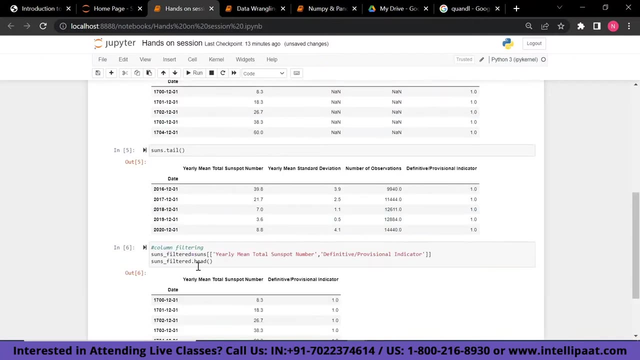 So I have created another variable called suns filter and then in this Pandas data frame, I have selected the columns which I wanted to see, such as yearly mean total sunspot number, yearly mean total sunspot number, yearly mean total sunspot number and definitive provisional indicator. and now I am printing the first five elements of these Pandas data frame. 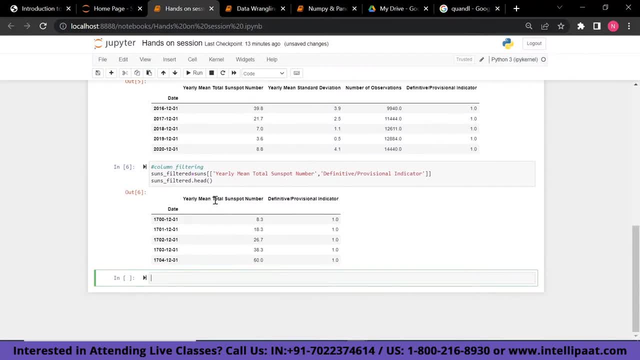 Let's run and see what happens Now. earlier you can see, we had one, two, three and four columns and now our columns are reduced and kind of filtered. So that's called, basically, column filtering, and we are performing this operations with the help of Pandas data frame which we have imported all around here. 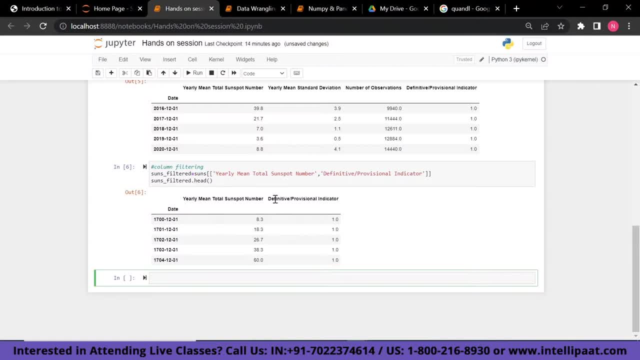 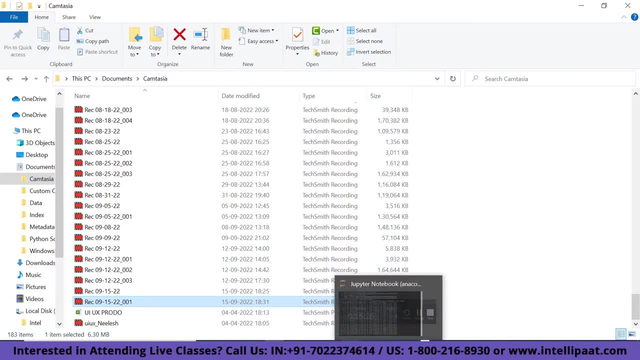 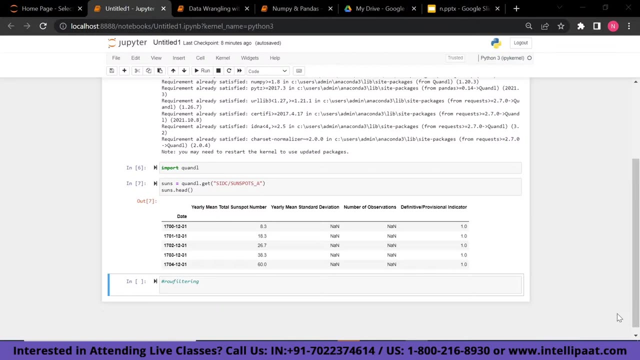 So we have filtered our column: yearly mean, total sunspot number and definitive provisional indicator. Now let's perform the next operation. that's called rows filtering. So now we are going to perform the row filtering. Pandas offers the ability to select rows. 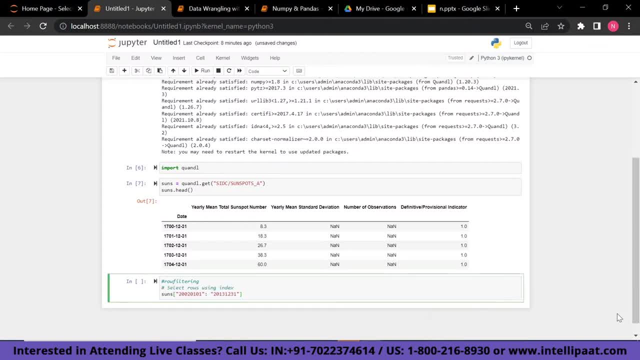 Let's select rows in a Pandas data frame. As you can see, I have selected the rows with the index of year. it's showing that 2002 to 2013.. Now I am going to display all the rows with the respective columns, from 2002 to 2013.. 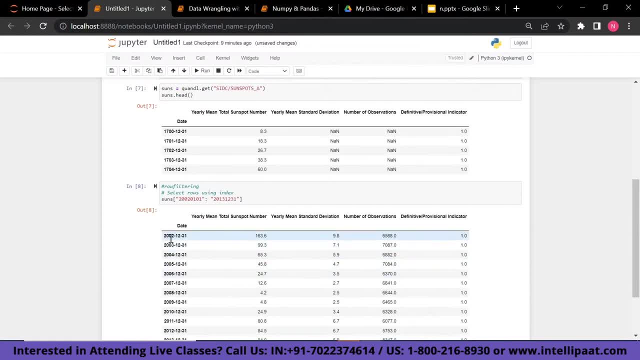 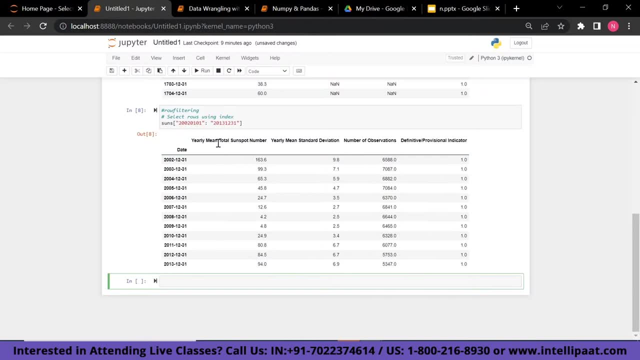 Let's run and see what happens to our filtering. You can see that our dates are coming from 2002 to 2013 and our column names are as follows. You are getting yearly mean total sunspot number, yearly mean standard deviation, number of observations and definitive and provisional indicator. 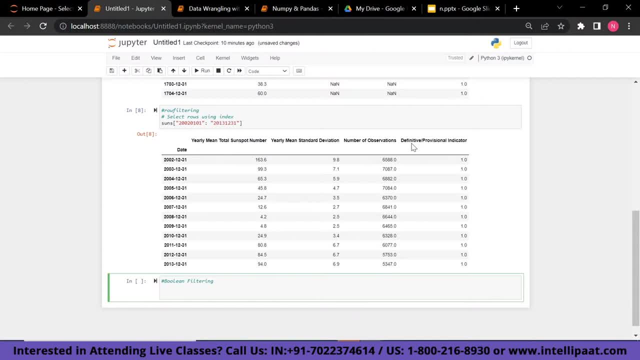 Now let's do the Boolean filtering. As you know, similar to the SQL via clause condition, we can query data using the Boolean conditions. Let's look at the data that is greater than the arithmetic mean. So, as you can see, I have written that suns bracket, suns, then again a bracket in which I am saying the column name and accessing the value of yearly mean total sunspot number, which is this. 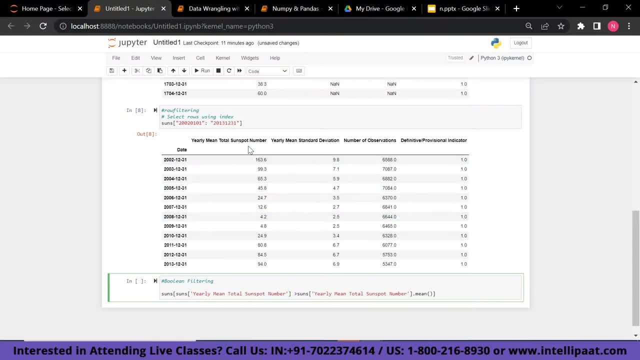 So I am accessing these values that are greater than the mean of these values. Okay, So how many value I want to filter it out as whose mean is greater than this yearly mean total sunspot number. So now let's perform the Boolean filtering. 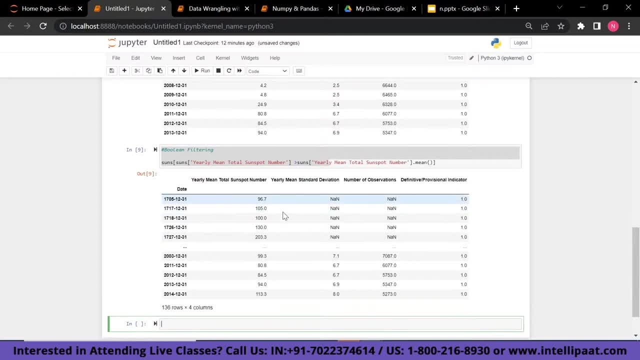 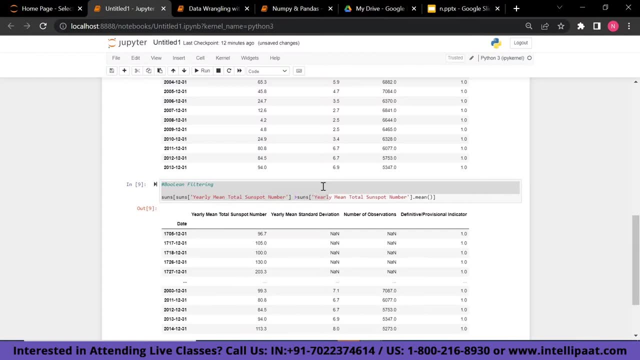 I will run it So you can see we are getting the column values. for the same, you know where I'm getting the values of the yearly mean total sunspot number, which is greater than the mean of the same column. So we are getting these values on the respective dates. 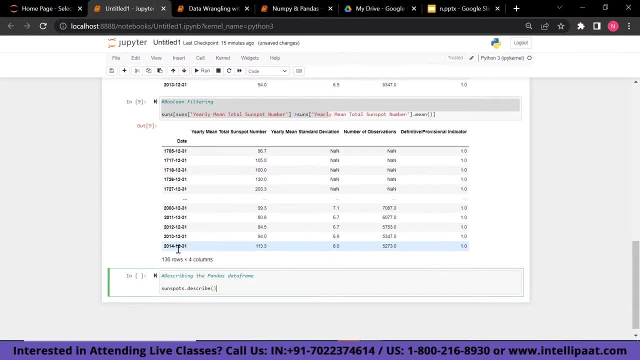 Now let's describe the Pandas DataFrame. So so, for the same purpose, I have used the describe method. Let me tell you something about the describe method. This method will show most of the descriptive statistical measures for all the columns in which I will gonna run it and then show you what are the parameters we are getting. 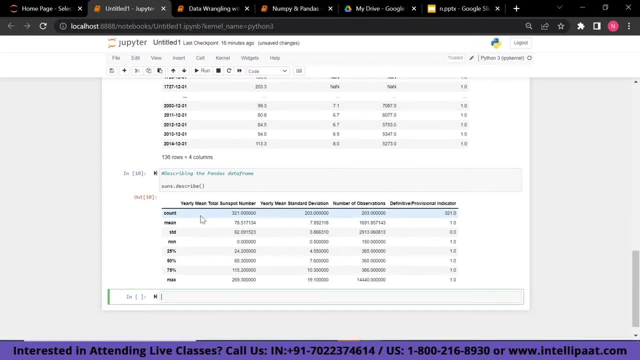 So since I have written sunsdescribe, which was our data frame so you can see for each of the respective columns, I'm getting count: mean standardization: minimum: 25 percentile, 50 percentile, 75 percentile and max. 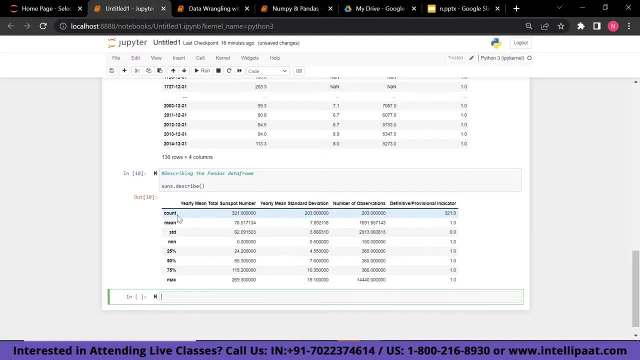 Let me tell you each one about them. First, let me talk about the count. The count method counts the number of observations in each column. It helps us to check the missing values in a data set. Except for the first three initial columns, all columns actually can have a missing value. 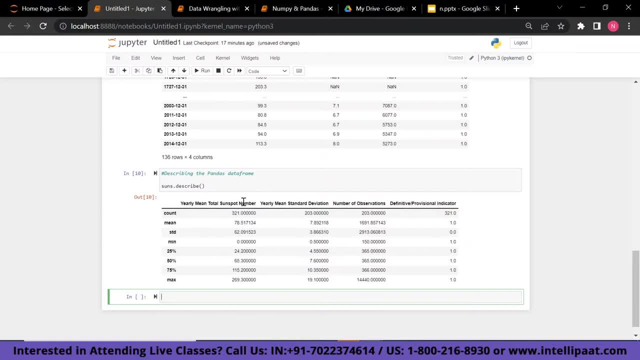 So, similarly, you can compute the median standard deviation, mean, absolute deviation, variance, skewness and kurtiosis. Next we have mean, which is used to give the mean for the respective columns. Then we have standard deviation, which also gives the respective standard deviation for each of these columns. 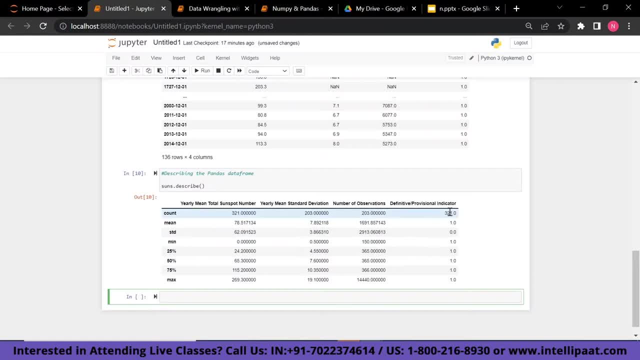 Then we have minimum value, which prints out the respective minimum value for each of the columns. Next we have 25 percentile, so it gives of the value of the 25 percentile of the data set, Similarly, the 50th percentile of the value we are going to get for the respective columns. 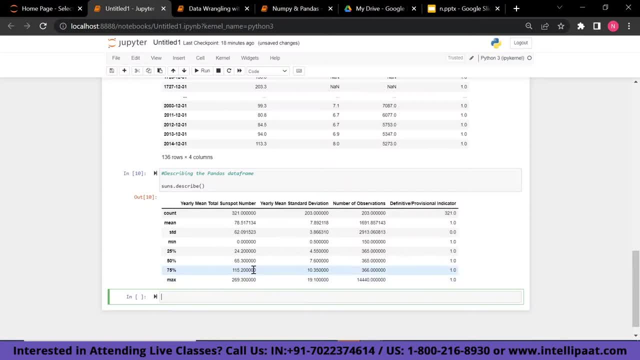 Similarly 75, and next it gives us the maximum value for each of the column. So this is all the things which is shown by the describe method. So we can say we are using the describe method of the pandas data frame in order to describe these things for our respective column. 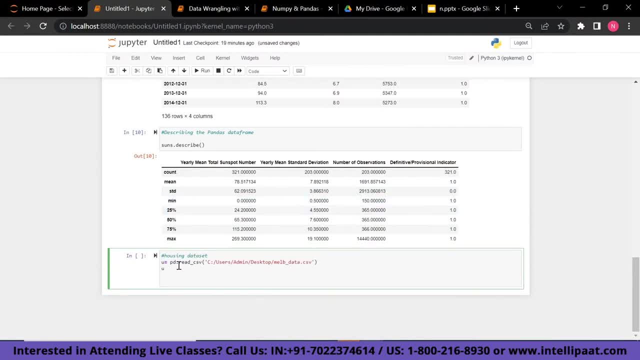 Now I am going to use the next data set, that is basically the housing data set of the Melbourne street, Then I am going to import that data set and then I am going to show you the group by operation. So, as you can see, I have imported our housing data set. 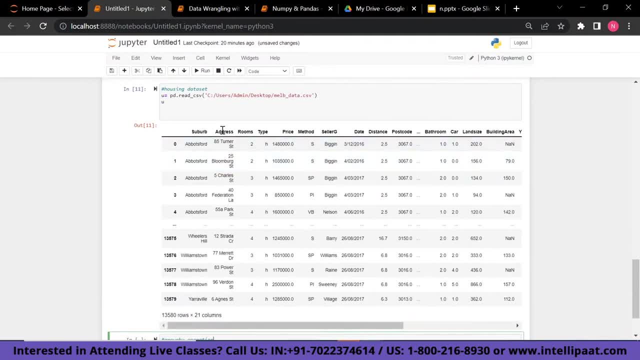 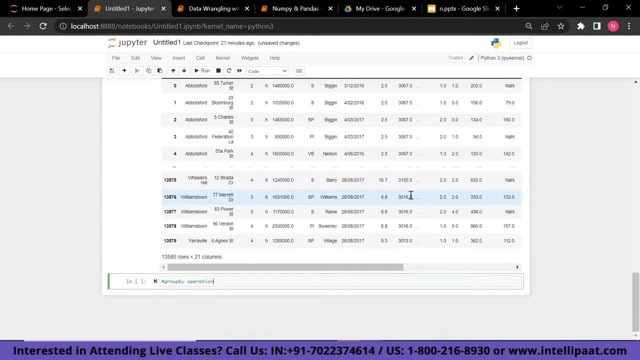 So you can see, we have columns such as suburb address, rooms type, price method, cellogy distance and so on. Now let me tell you something about the grouping operation. A grouping operation is a type of data aggregation operation. 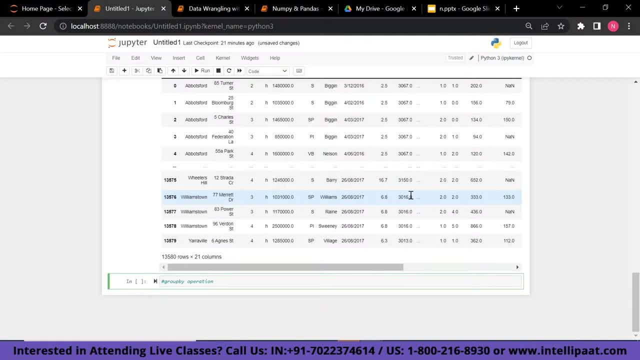 The term for grouping comes from the relational database To group similar types of values in a column. relational database software employs the group by operation. Now let me show you the group by keyword. Aggregate functions such as mean, min, max, count and sum can be applied to groups. 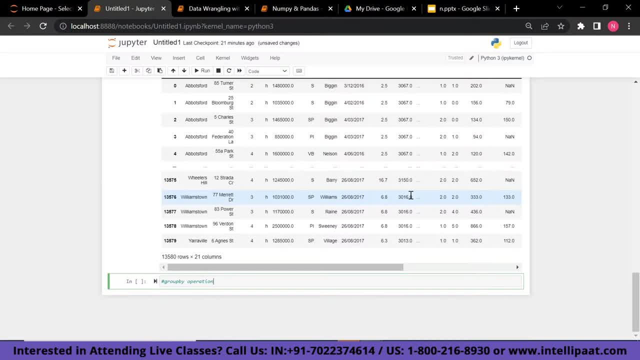 Similar capabilities are provided by the pandas data frame. The split apply strategy is used to apply the grouping operation. It divides data into groups, then applies aggregate operations such as mean, min, max, count and sum to each group and combines the result. Now let me show you the syntax for the group. 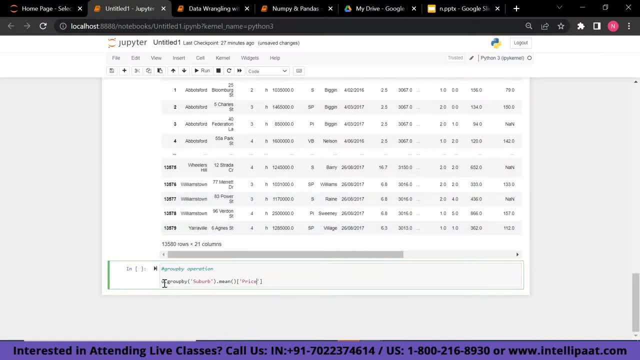 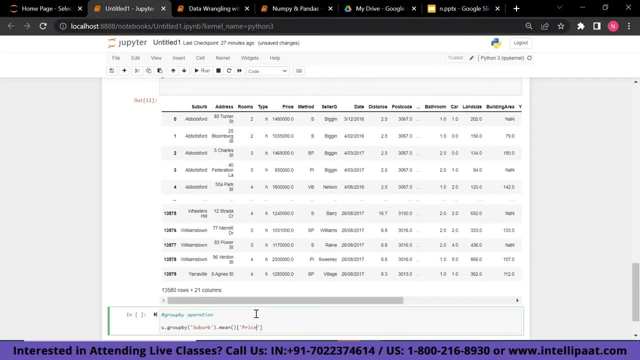 The group by operation. So I have selected our data frame, which we have imported right now, Then I am selecting the column called suburb, Then I am performing the mean operation on price. So basically for the respective suburbs I am going to get the mean price or the mean column for the same. 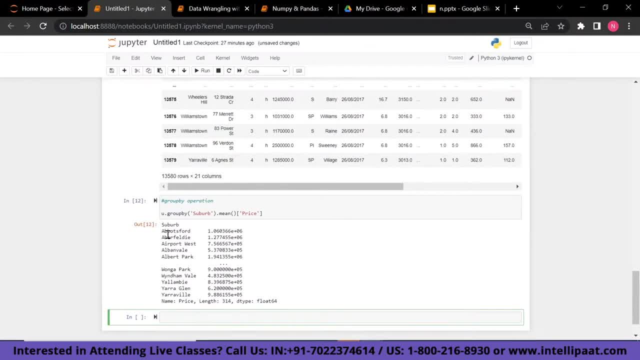 Let me run it and show you the result. So for respective suburbs we have Abbotsford, Aberfeldy, Airport West, So we are getting the respective price for the same. You can also see our results are coming in kind of an exponential form. 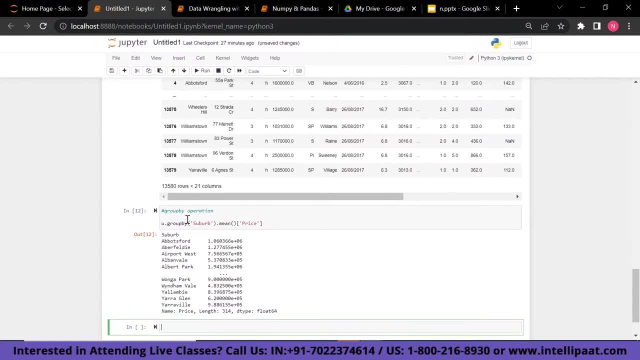 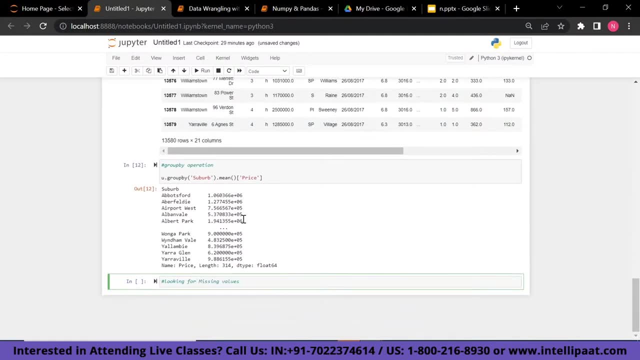 Similarly, you can perform a group by operation, in which you can take a column and use an aggregate function against another numerical column. Now the next thing, what we are going to do, is we are going to look for the missing values. So let me elaborate to you how we can look for the missing values. 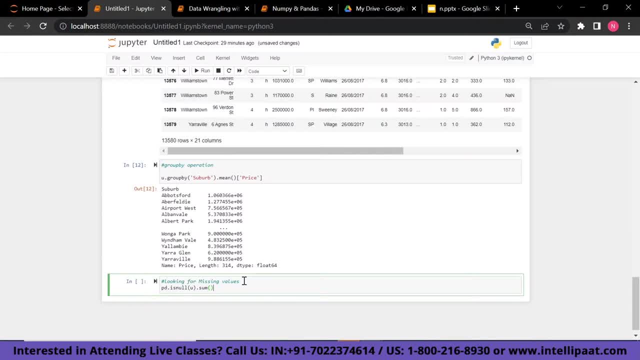 In the data frame for looking the missing values. pandas isNull function checks for the existence of null values And returns true or false where true is for the null and false is for the not null values. The sum function adds all the true values together and returns the number of missing values. 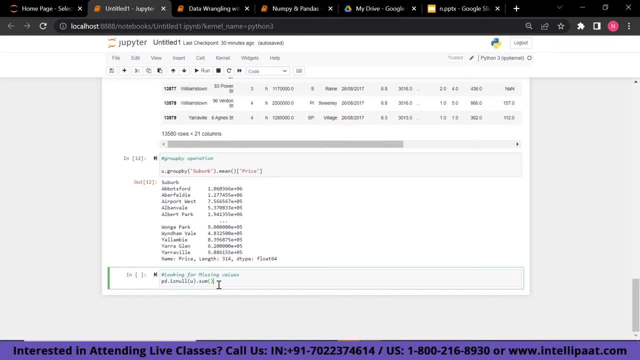 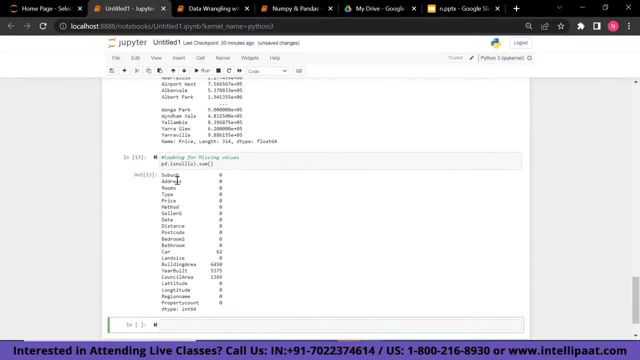 We are going to use these two methods for counting the number of missing values. Now let's run our cell and see the output. So for the respective columns we are getting 00. So in the column called suburb. So we have 0 missing values. 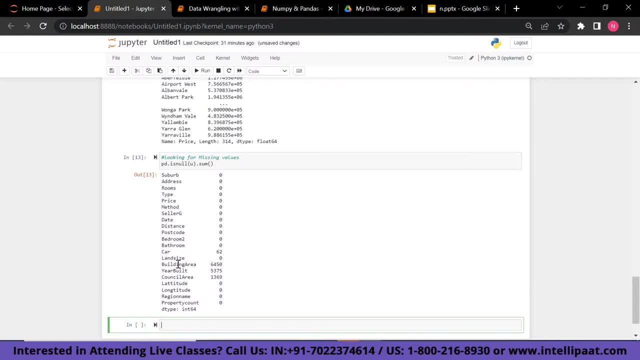 Similarly, for address, we have 0. But we have seen certain numbers In the columns, such as car building area, year built and council area. So these number of missing values we have. Now we are going to drop all the missing values. 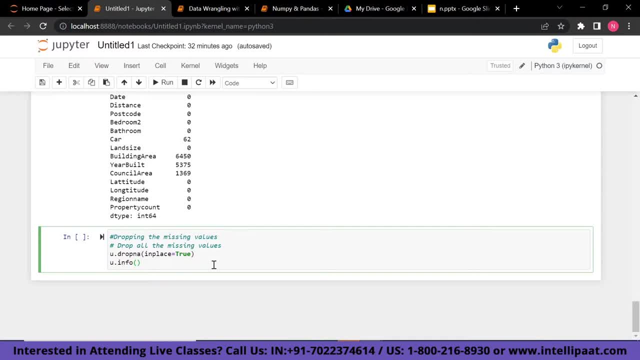 Dropping the missing values for the analysis purposes is kind of a very naive approach to deal with the missing values. The dropNull function in pandas can be used to drop or delete such observations from a data frame. The inplace equals to true attribute makes the following changes to our original database: 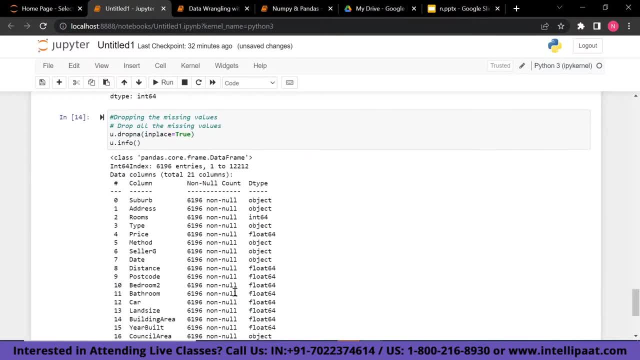 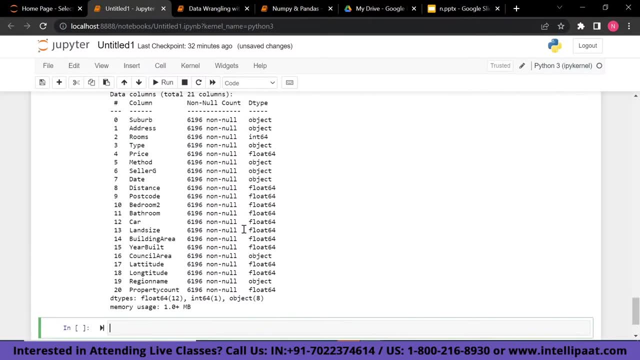 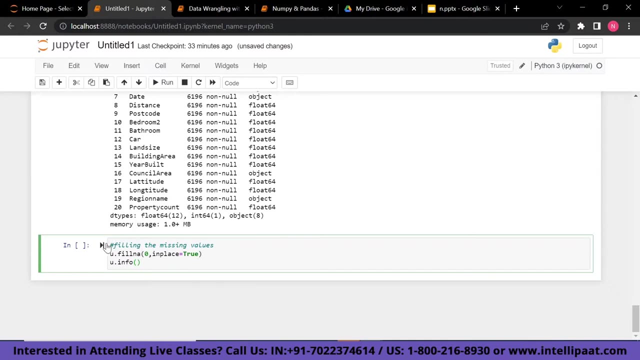 Now let me run the cell and show you, So you can see, that all our missing values have been dropped. You can also do one thing which I will show you: You can fill the missing values. So sometimes you can also handle the missing values by this way. 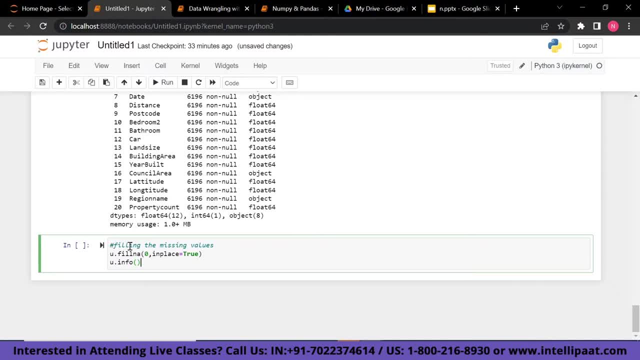 In which you are going to use the fillNull functions of the pandas and you can replace all the values with a 0 where the values are not present, And similarly, I have used the attribute inplace equals to true And I have printed uinfo, where u is our data frame. 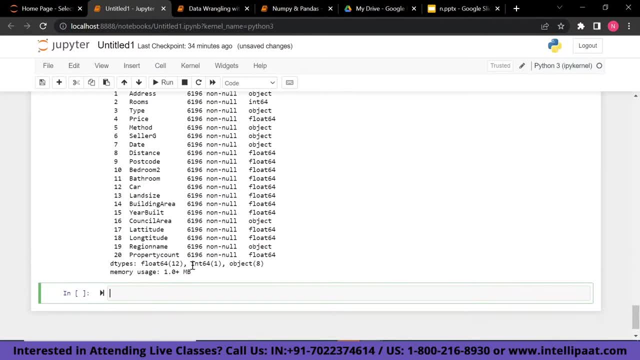 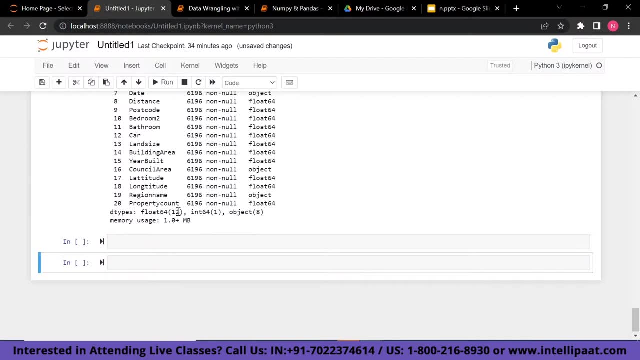 Let me run the cell and show you the output. You can see that our result is printed something like this: Now I am going to run it and show you that we have 0 null values present. So I am going to use the same function- pdisNull- and sum function to show you that we have 0 missing values. 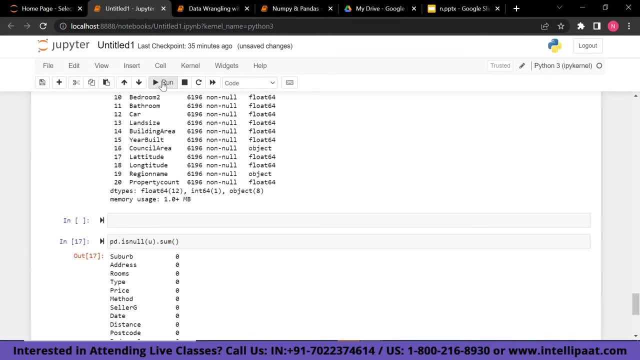 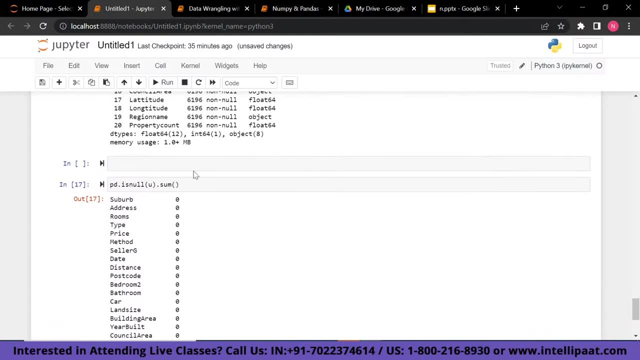 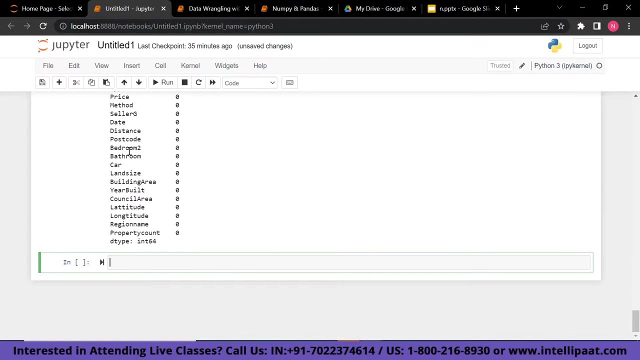 So let me run it and show you the output. You can see for our respective columns. we have 0 null values, Because all the null values or the missing values have been replaced by 0, which we have used there. Now let's move on to the next topic, which is developing the pivot table. 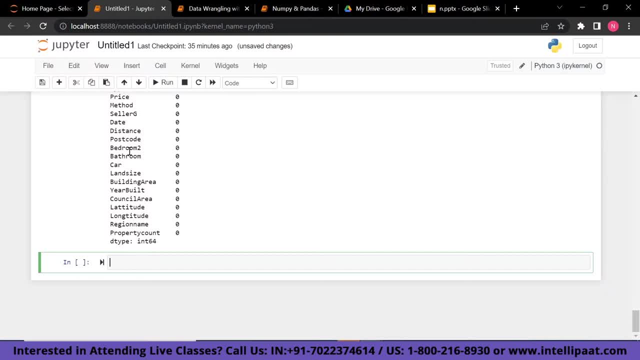 So I am going to show you how you can make a pivot table Now. before that, let me explain you what is basically a pivot table. A pivot table is essentially a summary table. It is the most widely used concept in Excel. Most data analysts use it as a convenient tool to summarize their findings. 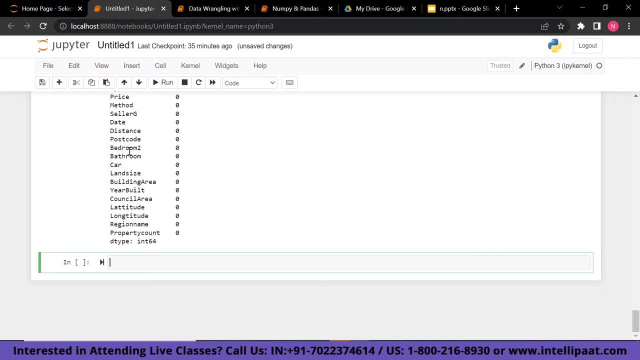 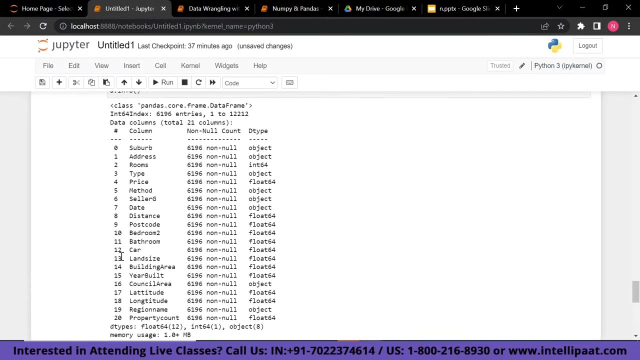 To summarize data frames. pandas provide the pivot table function. An aggregate function, such as min, min, max or sum is used to summarize the data frame. Now we will summarize the data frame using the following code. So now, first let me show you how is our original table. 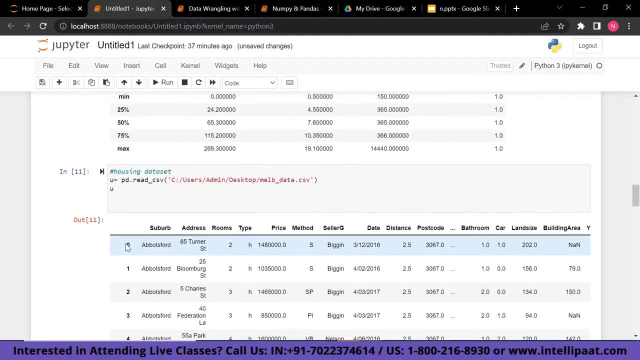 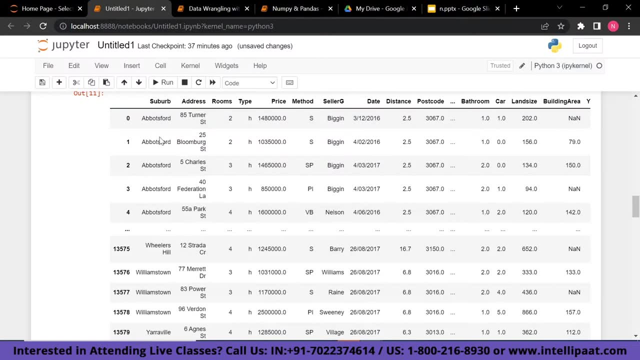 So I have used all over here. So you can see this is our original table. Now our target here is to create a pivot table. So for the index of suburb, I am going to print the respective prices. Okay, 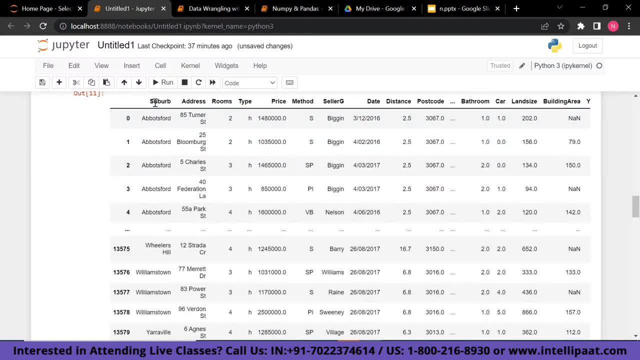 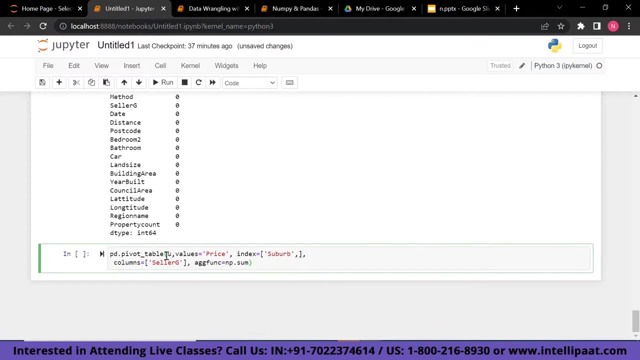 And we have seller g's. So here we will have all the suburbs and here we are going to have all the sellers, such as Bigin, Bigin, Nelson, Barry, and respective prices for our suburb is going to get printed. So for the same thing I have done all over here that I have used our data frame, which is u. 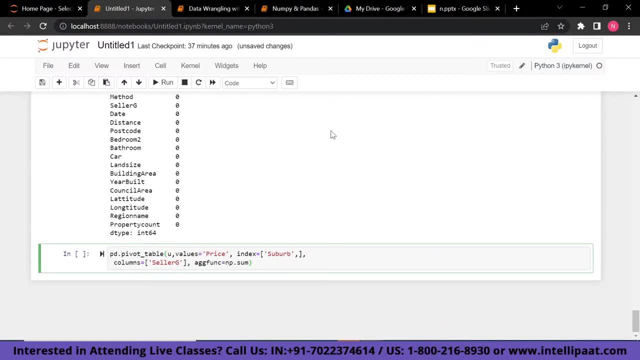 and I have used the values called price, So in the index it will be suburb and the columns we are going to get the seller g, And I have used an aggregate function called npsum. Let me print this cell and show you how the results are coming. 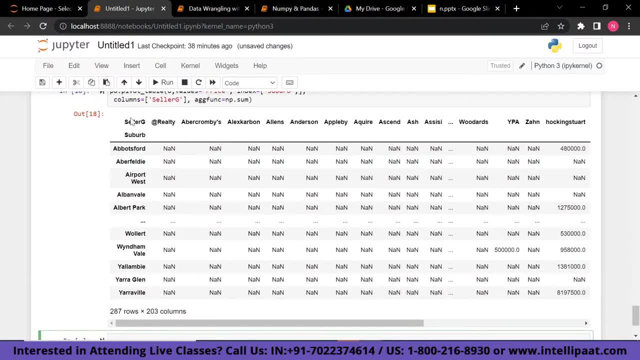 So you can see all over here that here in this column we have all the sellers, such as Realty Abercrombie, Allens Anderson, Applebuy and similarly, And here we have all the suburbs all over here. So and respective prices are print if they are present in our data set. 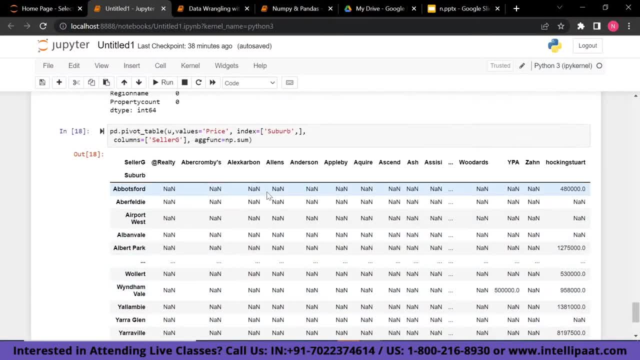 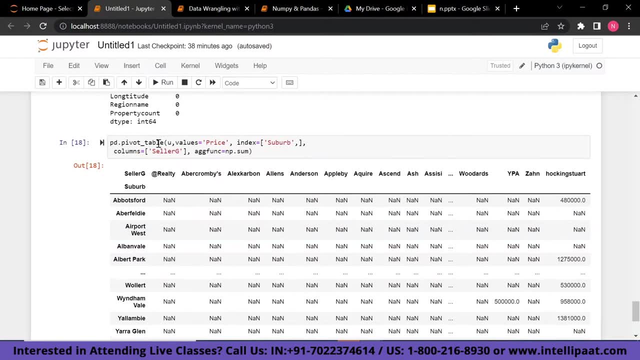 So you can consider this as a pivot table. Okay, I hope so. you have got an idea how to create a pivot table. So, similarly, you are going to use a pivot table. You are going to use a pivot table function all over here. 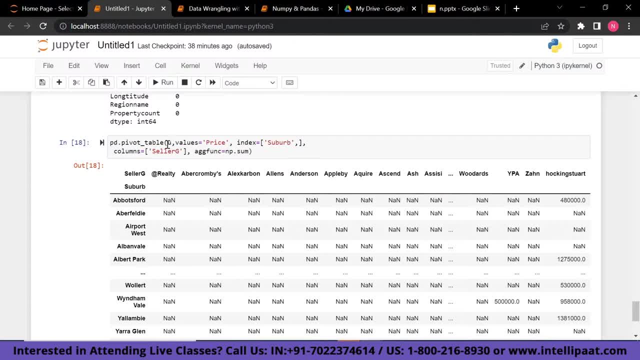 So you are going to use pdpivotTable, Then you are going to close the parenthesis with u, Then you are going to use the attributes, such as value, index and column, And the next attribute you can also use is aggregate function, which you can use anything, such as mean, min, max or standard deviation. 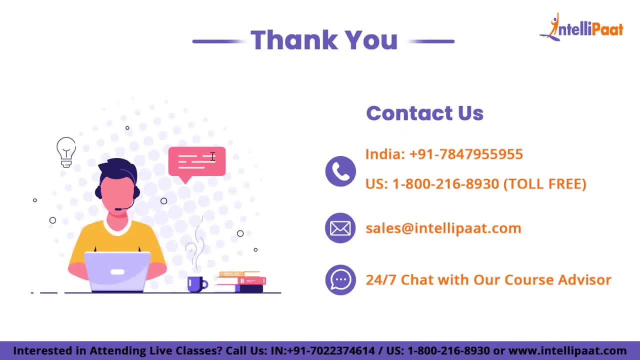 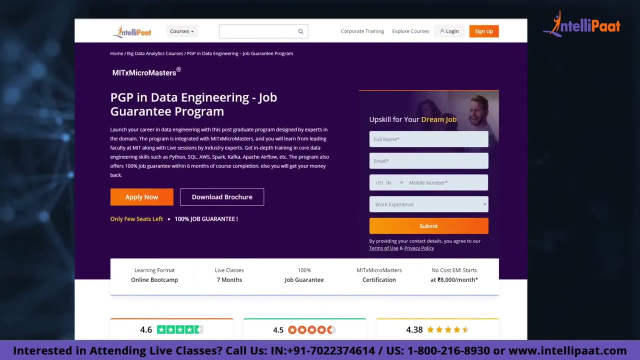 That was all for this session. I hope so you would have enjoyed our session on data wrangling and also enjoyed the hands-on session. Till then, keep learning. I will meet you in the next session. Just a quick info, guys. If you want to learn data engineering, then Intellipaat provides a job guarantee program. 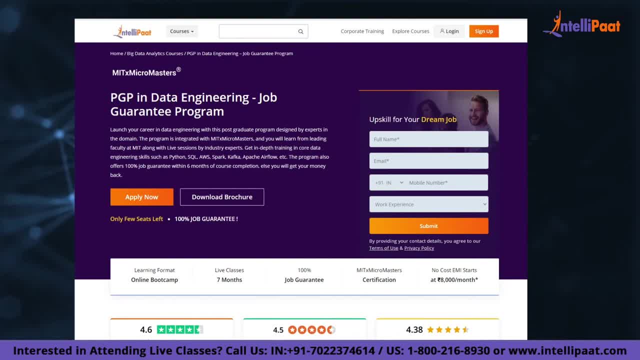 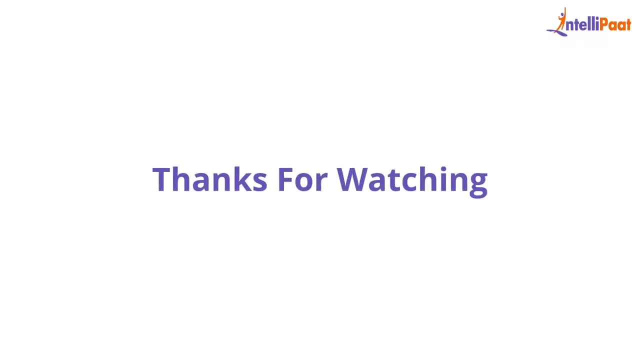 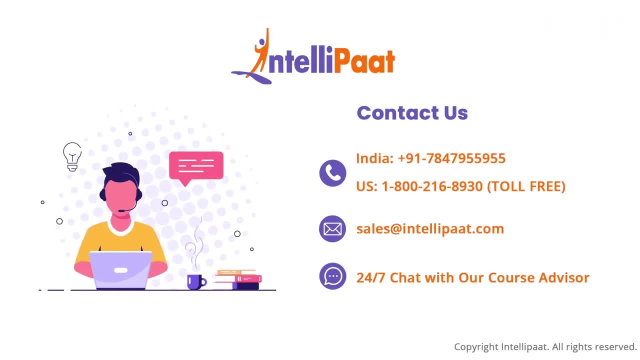 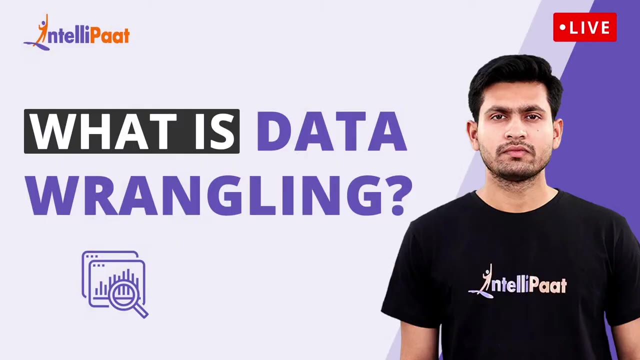 in collaboration with MIT MicroMasters. This course will be taught by MIT professors and industry experts. This course will help you to upskill and land your dream job. Thank you, Thank you.